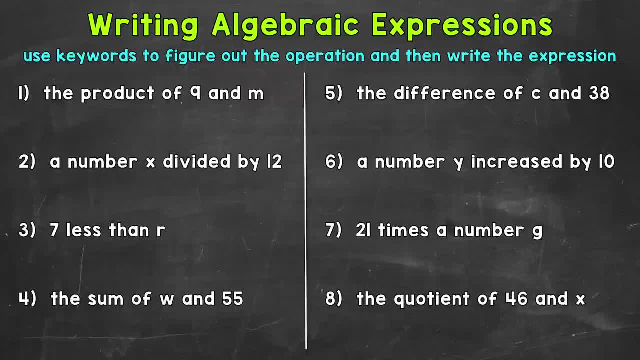 So product is going to be our key word. It means the answer to a multiplication problem. So we know this is going to be multiplication 9 times m. Now m is our variable. It's a letter that represents a value we do not know yet, so an unknown. Let's go through some different ways. 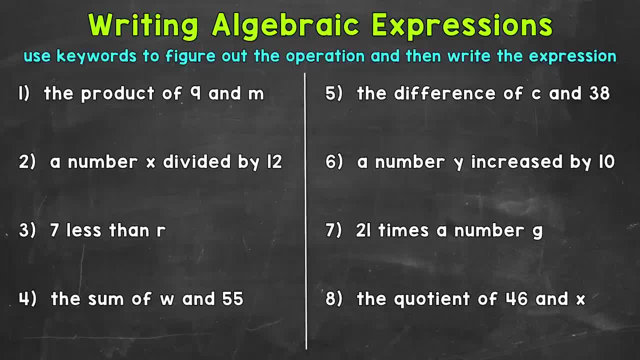 that we can write algebraic expressions that involve multiplication. Now, this first one: we want to write algebraic expressions. So let's go through some different ways that we can write algebraic expressions that involve multiplication. Now, this first one: we want to write algebraic. 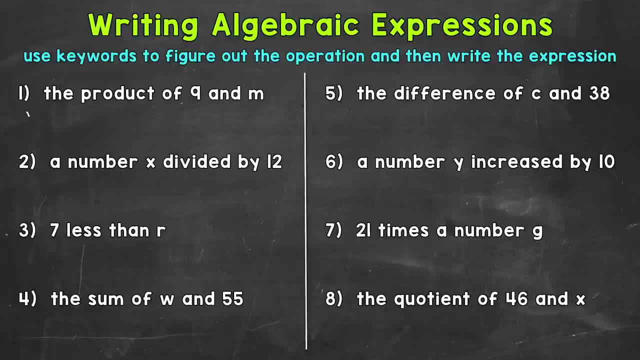 expressions that involve multiplication. Now, this first one, we want to write algebraic expressions to avoid, and that's using an x to represent our multiplication symbol. Now, we want to avoid this so we don't have any confusion, because this can mean two things: 9xm, where we have an algebraic 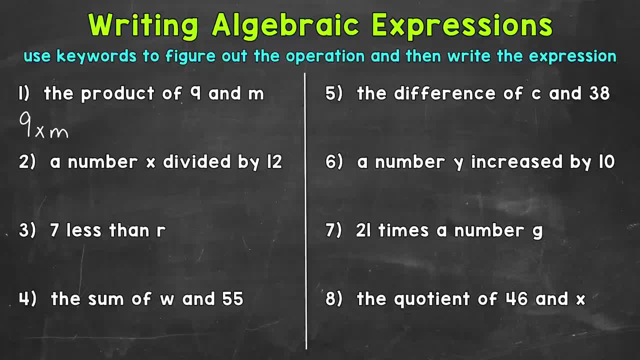 expression with two variables, x and m, or does it mean 9 times m? So let's avoid using that. Our other options, well, the first one we can use: 9m, So a number next to a variable. 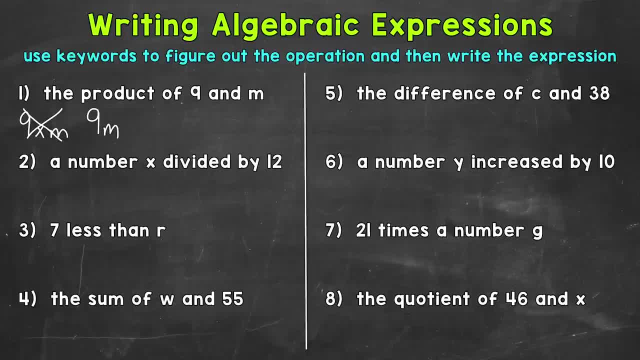 represents multiplication. Another option would be using an asterisk, So something that looks like this represents multiplication as well. Another option, using a filled-in circle or dot represents multiplication. And then, lastly, we can use parentheses, So anytime we have a. 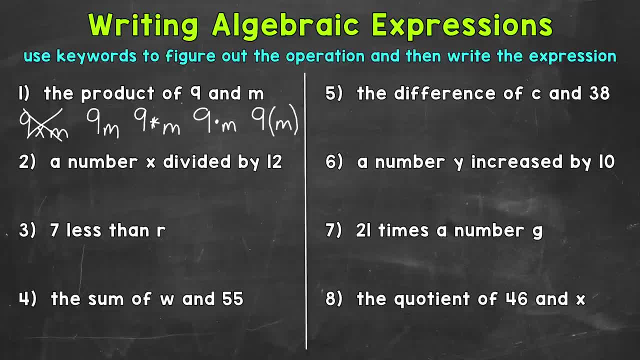 number next to parentheses. that represents multiplication as well. Let's move on to number two, where we have a number- x divided by 12.. So this is going to be division. So we can write this out: x divided by 12.. So this is going to be division. So we can write this out: x divided. 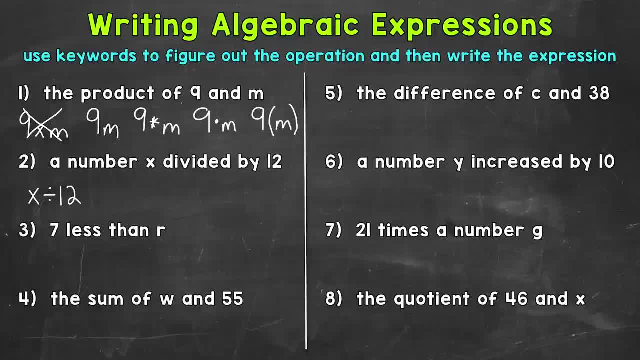 by 12.. We can do x divided by 12, or we can do a slash x divided by 12.. So some different options for division as well. Number three: 7 less than r. Now this one. we switch the order. 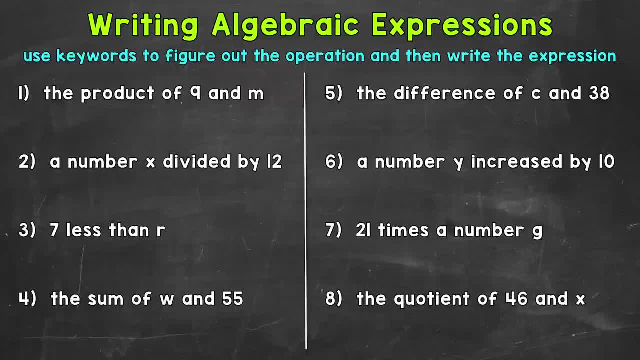 So product is going to be our key word. It means the answer to a multiplication problem. So we know this is going to be multiplication 9 times m. Now m is our variable. It's a letter that represents a value we do not know yet, so an unknown. Let's go through some different ways. 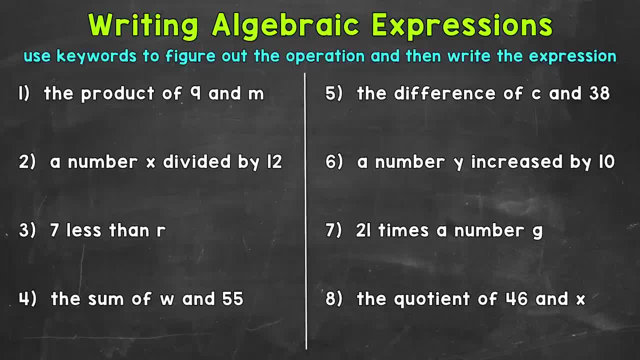 that we can write algebraic expressions that involve multiplication. Now, this first one: we want to write algebraic expressions. So let's go through some different ways that we can write algebraic expressions that involve multiplication. Now, this first one: we want to write algebraic. 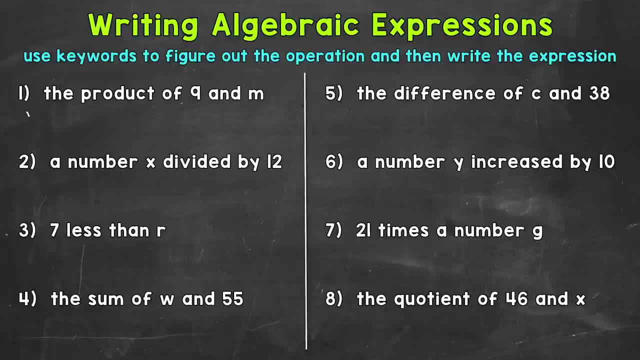 expressions that involve multiplication. Now, this first one, we want to write algebraic expressions to avoid, and that's using an x to represent our multiplication symbol. Now, we want to avoid this so we don't have any confusion, because this can mean two things: 9xm, where we have an algebraic 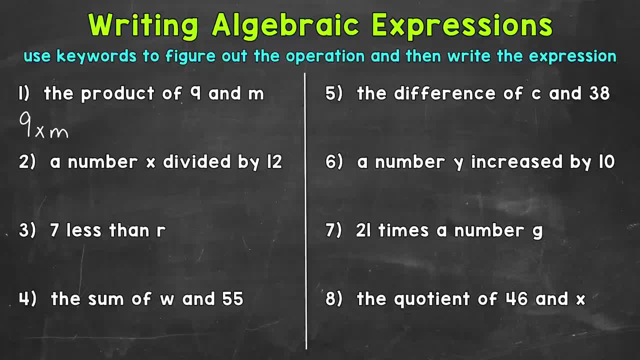 expression with two variables, x and m, or does it mean 9 times m? So let's avoid using that. Our other options, well, the first one we can use: 9m, So a number next to a variable. 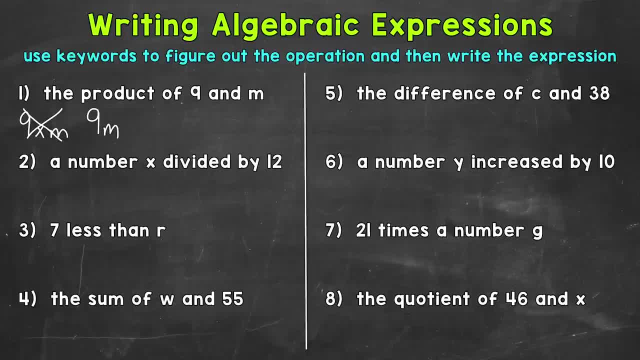 represents multiplication. Another option would be using an asterisk, So something that looks like this represents multiplication as well. Another option, using a filled-in circle or dot represents multiplication. And then, lastly, we can use parentheses, So anytime we have a. 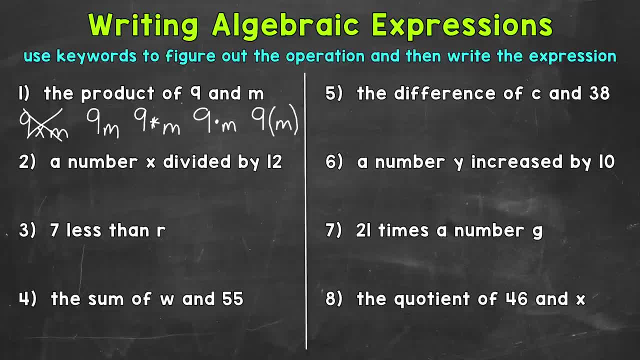 number next to parentheses. that represents multiplication as well. Let's move on to number two, where we have a number- x divided by 12.. So this is going to be division. So we can write this out: x divided by 12.. So this is going to be division. So we can write this out: x divided. 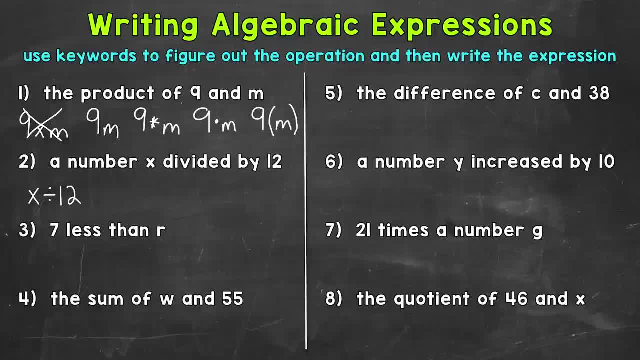 by 12.. We can do x divided by 12, or we can do a slash x divided by 12.. So some different options for division as well. Number three: 7 less than r. Now this one. we switch the order. 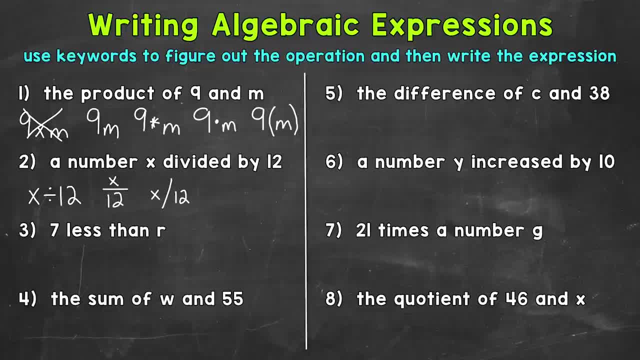 and we need to think less than. We are taking 7 less than r. So this is going to be subtraction and it's going to be r minus 7 less than So whenever we see less than, we actually switch the order. So the r comes first and the 7 comes second. We are 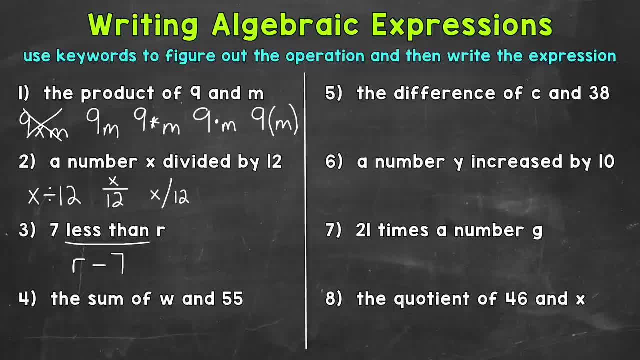 taking 7 less than that r. So switch that order. Number four: the sum of w and 50. So sum is our keyword there and that's the answer to an addition problem. So this is going to be addition w plus 55.. On to number five, where we have the difference of c and 38. So 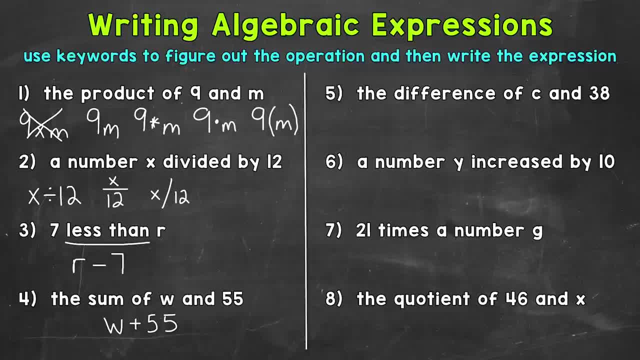 our keyword difference. well, that's the answer to a subtraction problem. So this is going to be subtraction c minus 38.. So in the case of that subtraction algebraic expression we keep the order c first, 38 second, as opposed to number three where we switch that order. That's because 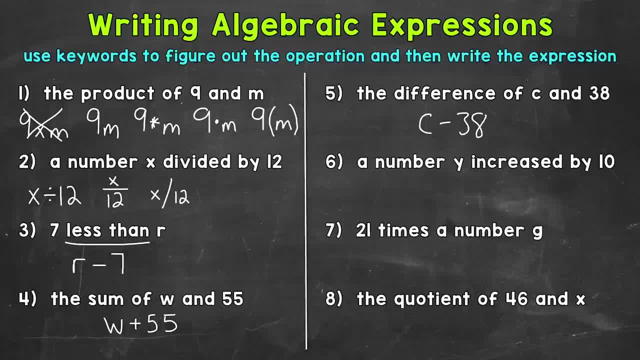 we had that less than So pay attention to wording when it comes to these algebraic expressions. number six: we have a number y increased by 10. increased is our keyword. that means that we are going to use addition, so y plus 10. on to number 7, 21 times a number g, so multiplication. so let's use 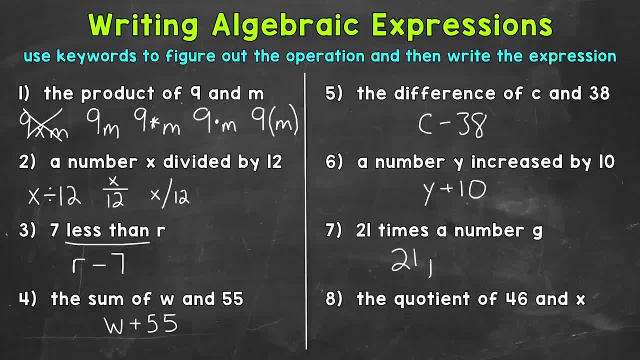 a number next to our variable. remember that represents multiplication. so 21 g represents 21 times g. lastly, number eight, the quotient of 46 and x. now, quotient is our keyword. it means the answer to a division problem. so this is going to be division 46 divided by x. 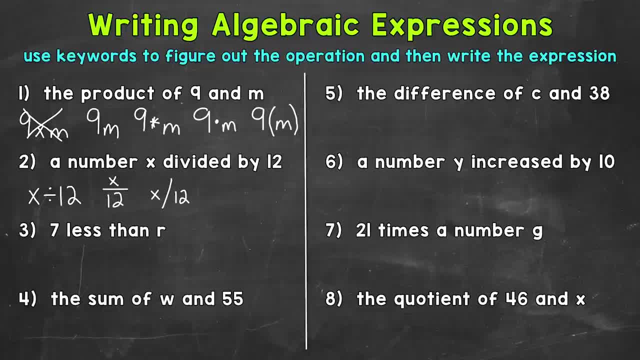 and we need to think less than. We are taking 7 less than r. So this is going to be subtraction and it's going to be r minus 7 less than So whenever we see less than, we actually switch the order. So the r comes first and the 7 comes second. We are 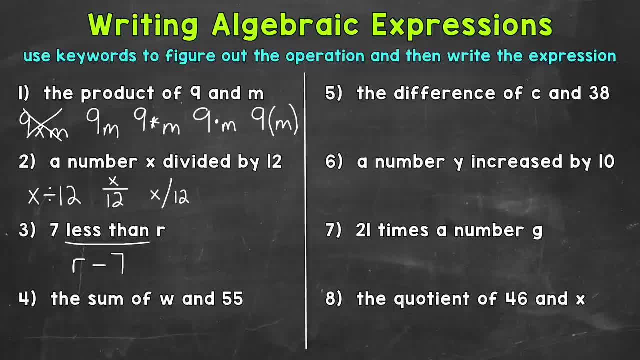 taking 7 less than that r. So switch that order. Number four: the sum of w and 50. So sum is our keyword there and that's the answer to an addition problem. So this is going to be addition w plus 55.. On to number five, where we have the difference of c and 38. So 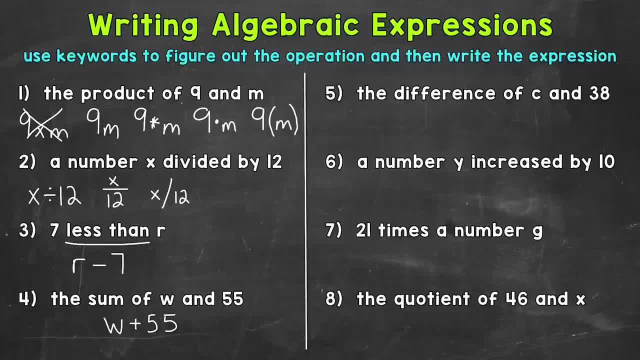 our keyword difference. well, that's the answer to a subtraction problem. So this is going to be subtraction c minus 38.. So in the case of that subtraction algebraic expression we keep the order c first, 38 second, as opposed to number three where we switch that order. That's because 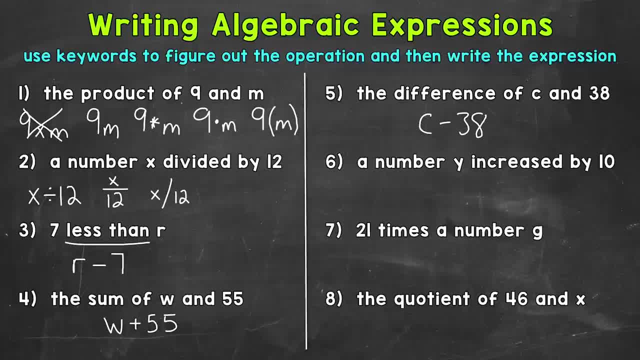 we had that less than So. pay attention to wording when it comes to these algebraic expressions. Number six: We have a number, Y, increased by 10.. Increased is our key word. That means that we are going to use addition, So Y plus 10.. 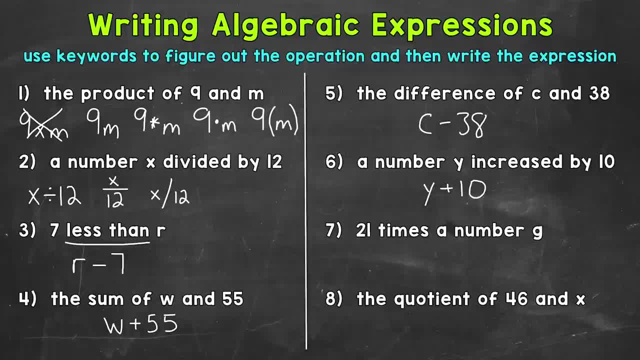 On to number 7.. 21 times a number, G, So multiplication. So let's use a number next to our variable. Remember that represents multiplication. So 21G represents 21 times G. Lastly, number 8.. The quotient of 46 and X. 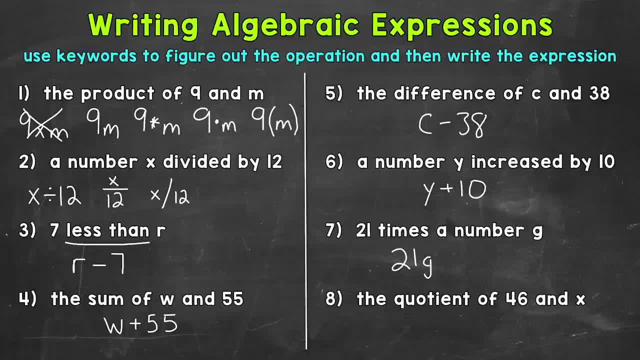 Now, quotient is our key word. It means the answer to a division problem. So this is going to be division 46 divided by X. So let's represent this using a fraction And this is a division problem: 46 divided by X. 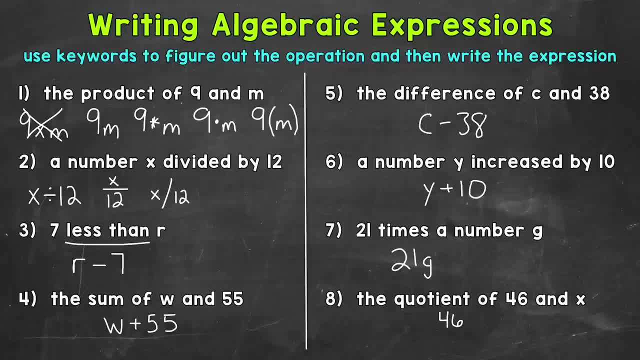 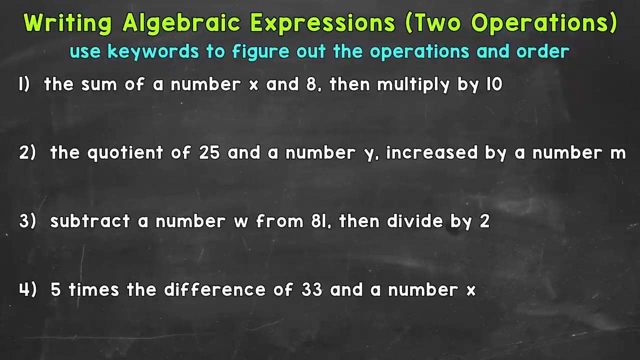 you. So let's represent this using a fraction, and this is a division problem: 46 divided by x. So there are some examples of writing expressions with one operation. Let's move on to some expressions with two operations. We will start with number 1, where we have the sum of a number, x and 8, then multiply by 10.. 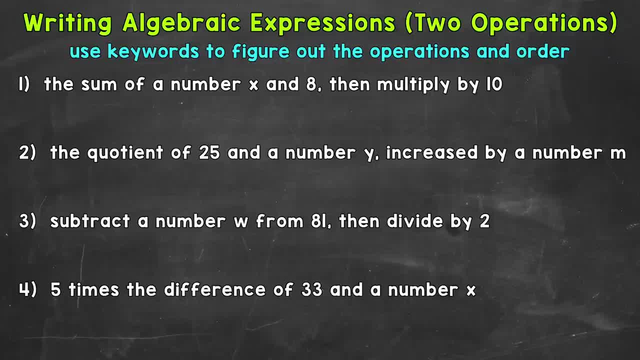 Let's break this down and figure out what we need to do first. And the first thing that we need to do is the sum of a number: x and 8.. Our keyword is sum. That means the answer to an addition problem. So we are going to add x plus 8.. 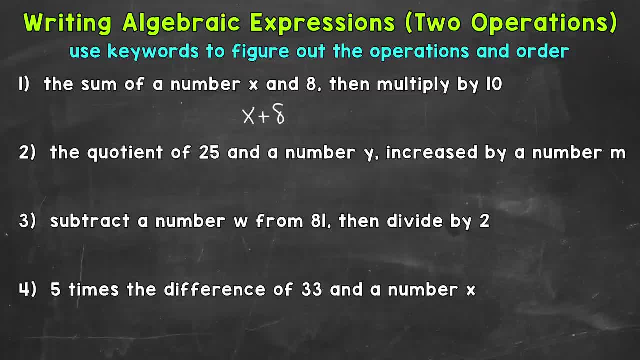 x plus 8.. I'm going to use parentheses to show that we have to do that first. So we are going to add x plus 8.. So we are going to add x plus 8.. Based on the order of operations. So use parentheses to show what you need to do first. 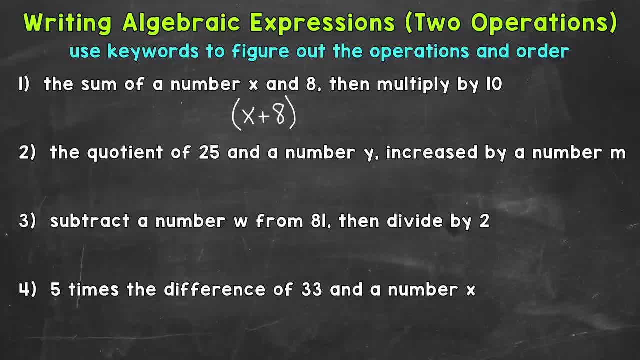 Now, secondly, we need to then multiply by 10.. So let's multiply by 10.. There are different ways to represent multiplication within algebraic expressions and math in general, So for this one I'm going to use the filled in circle or dot there. 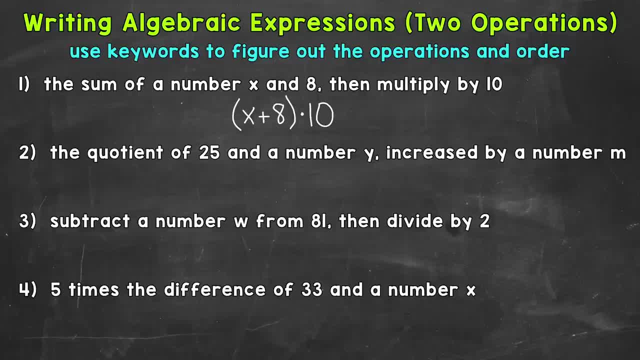 So x plus 8.. Within parentheses: times 10.. That would represent that phrase. Now we can also do. Let me rewrite this: x plus 8. Within parentheses, And the 10 can come first, Because the order of operations here. 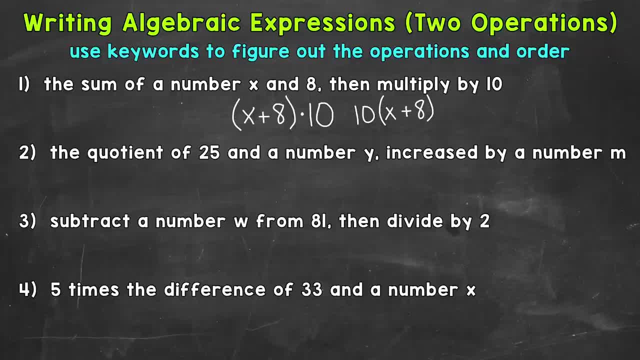 We would have to do the x plus 8. Within those parentheses, And then we would multiply by 10. And remember, anytime you have a number Next to parentheses It represents multiplication. So there can be more than one correct answer for these algebraic expressions. 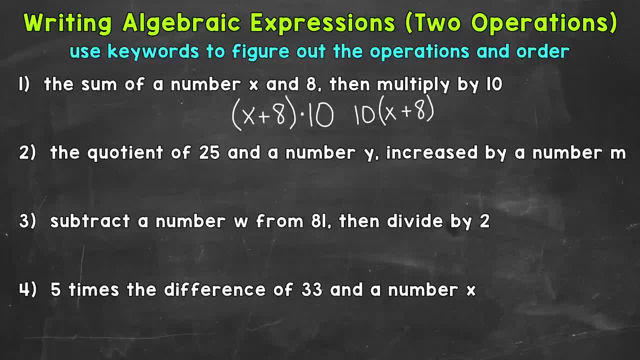 Now one incorrect answer for number one that I want to show you Would be x plus 8. And then multiply by 10. This would be incorrect because of the order of operations. We would have to do multiplication first. So we would have to do multiplication first. 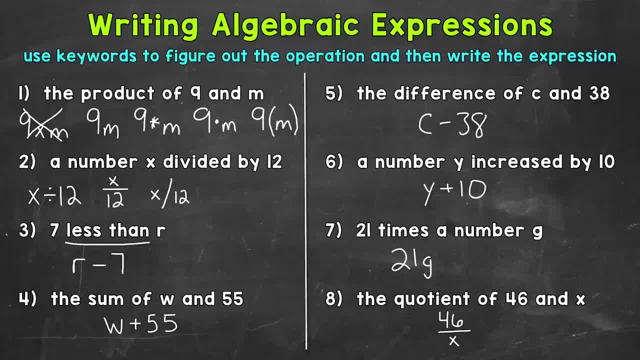 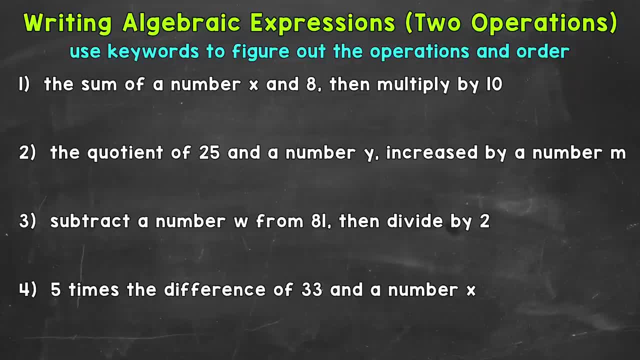 So there are some examples of writing expressions with one operation. Let's move on to some expressions with two operations. We will start with number 1, where we have the sum of a number X and 8, then multiply by 10.. Let's break this down and figure out what we need to do first. 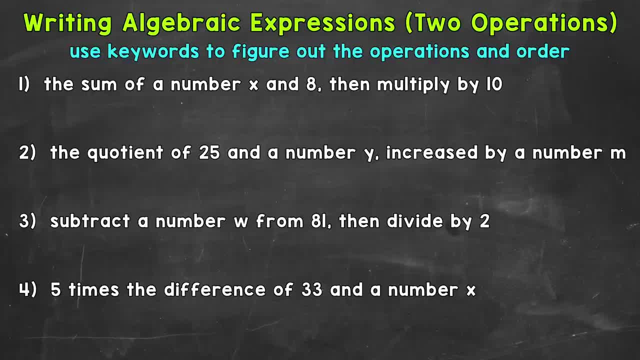 And the first thing that we need to do is the sum of a number: X and 8.. Our key word is sum. That means the answer to an addition problem. So we are going to add X plus 8.. X plus 8.. 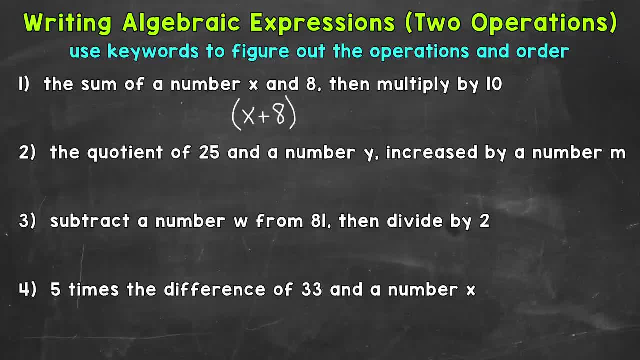 I'm going to use parentheses to show that we have to do that first, based on the order of operations. So use parentheses to show what you need to do first Now. secondly, we need to then multiply by 10.. So let's multiply by 10.. 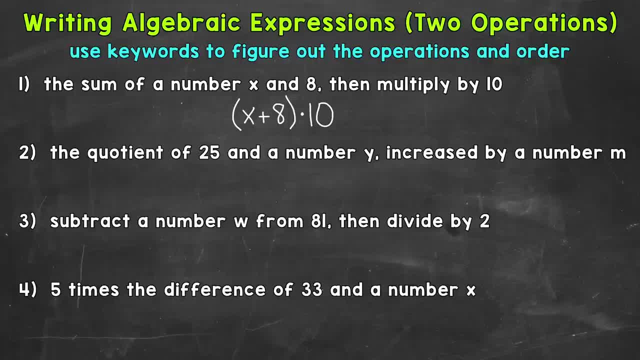 There are different ways to represent multiplication within algebraic expressions and math in general, So for this one I'm going to use the filled in circle or dot there. So X plus 8, within parentheses, times 10.. That would represent that phrase. 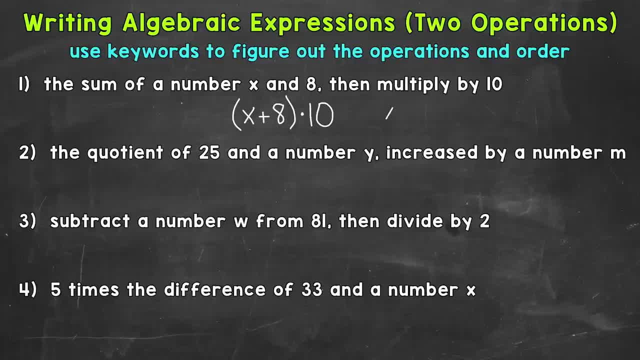 Now we can also do. let me rewrite this: X plus 8 within parentheses, And the 10 can come first, because the order of operations here we would have to do the X plus 8 within those parentheses And then we would multiply by 10.. 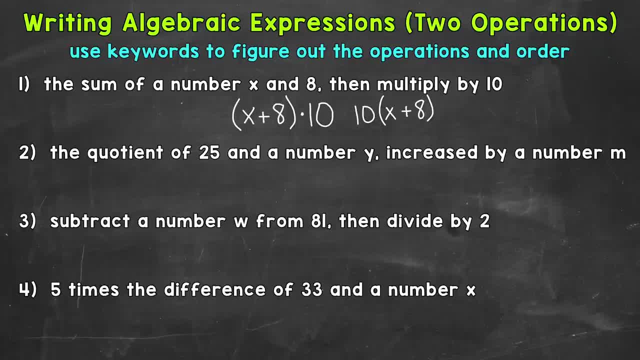 And remember, anytime you have a number next to parentheses, it represents multiplication, So there can be more than one. So that's the one correct answer for these algebraic expressions. Now one incorrect answer for number one that I want to show you would be X plus 8.. 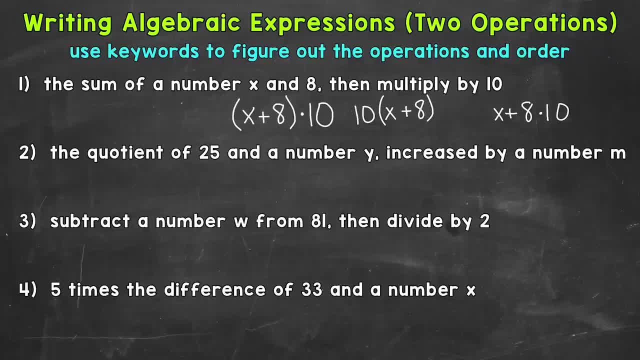 And then multiply by 10.. This would be incorrect because of the order of operations. We would have to do multiplication first, So we would have to do 8 times 10 and then add X. X plus 8 has to be within the order of operations. 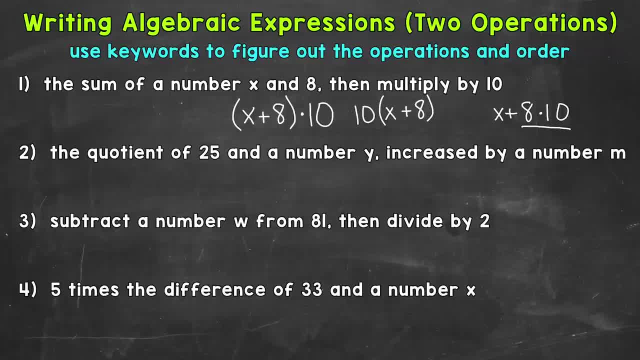 So we would have to do 8 times 10 and then add X. So we would have to do 8 times 10 and then add X. So we would have to do 8 times 10 and then add X. Let's move on to number two. 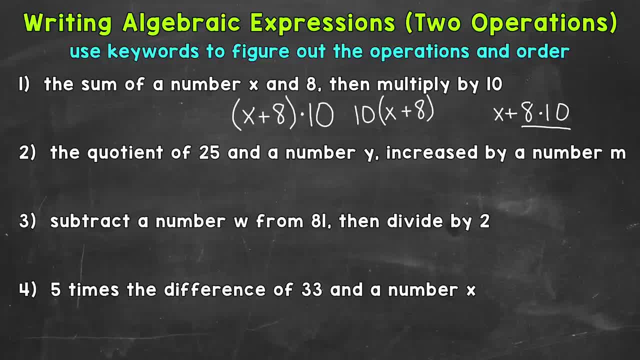 We would have to do 8 times 10. And then add x. x plus 8 has to be within parentheses In order to show that that's what we do first. So something to keep in mind there. Let's move on to number two. 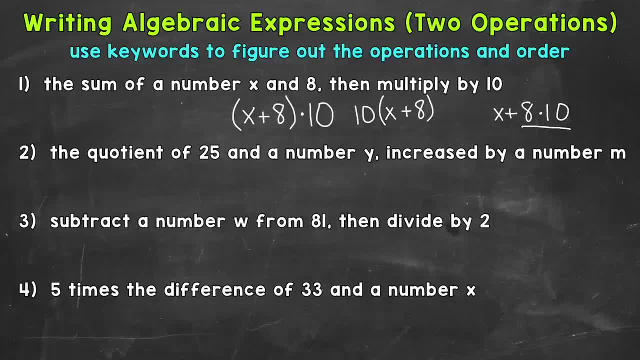 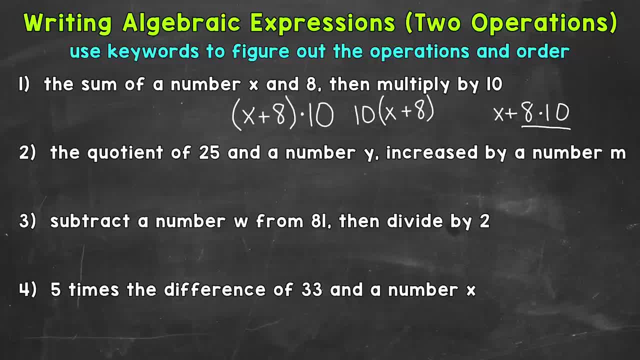 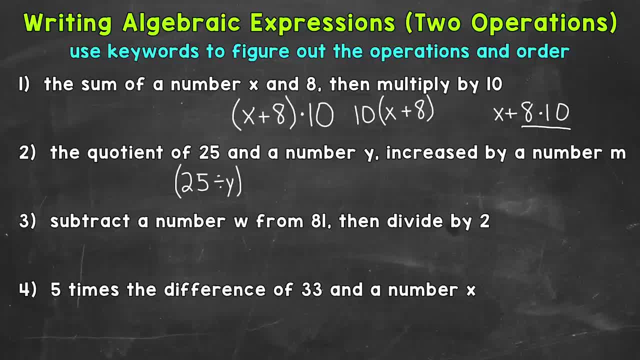 To show that that's what we do first. I also want to mention that there are other ways to represent division as well, Such as writing the division problem As a fraction Or using a slash, So we have the quotient of 25.. 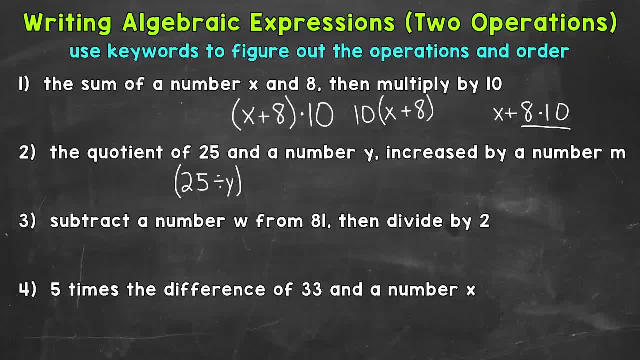 And a number y represented. Now we need to do our second step, Which is increased by a number m. Increased is our key word, And this means that we are going to add m. So plus m, And that's our algebraic expression. 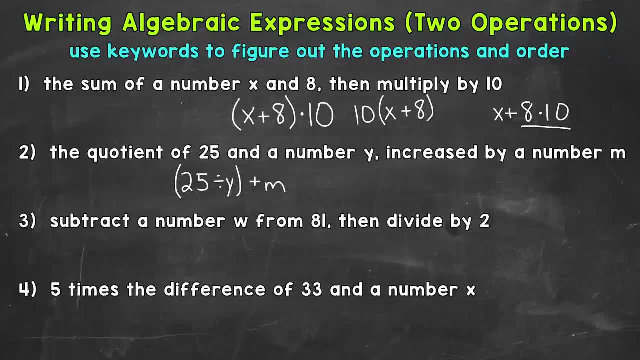 We can also write it without Parentheses, though, Because, due to the order of operations, We need to do division before addition. So 25 divided by y Plus m Would be correct as well, Again because due to the order of operations. 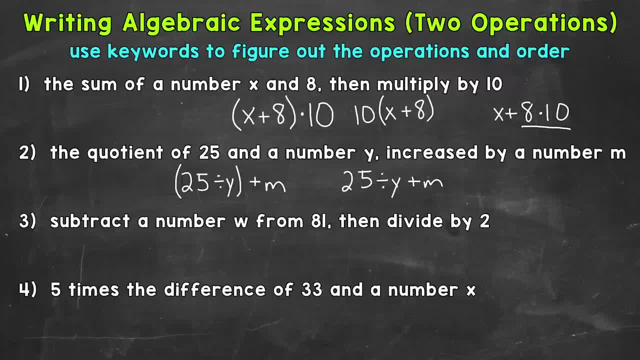 We need to do division before addition, So we would have to do 25 divided by y First and then add m. Let's move on to number six, Number three, Where we have subtract a number w from 81. Then divide by two. 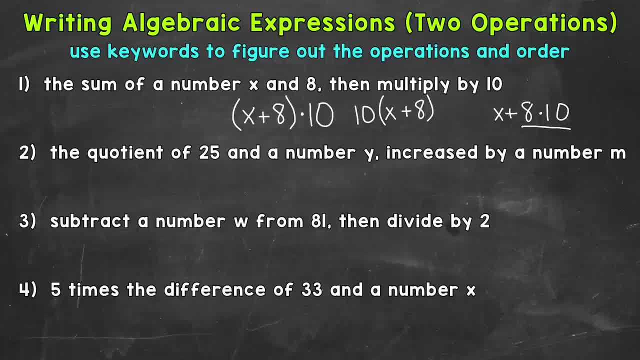 where we have the quotient of 25 and a number Y increased by a number M. Let's start with the quotient of 25 and a number Y. Quotient is going to be our key word. It means the answer to a division problem. 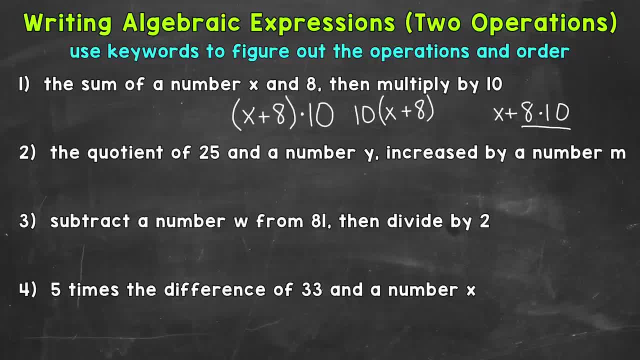 So we are going to do So. we are going to do 25 divided by Y. So 25 divided by Y, And I'm going to put this within parentheses to show that that's what we do first. I also want to mention that there are other ways to represent division as well. 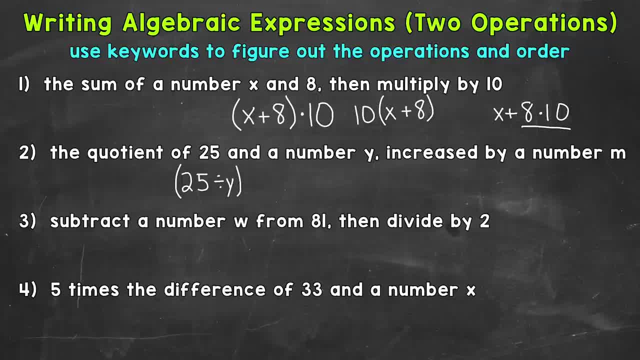 such as writing the division problem as a fraction or using a slash. So we have the quotient of 25,. So we have the quotient of 25, and a number Y represented. Now we need to do our second step, which is increased by a number M. 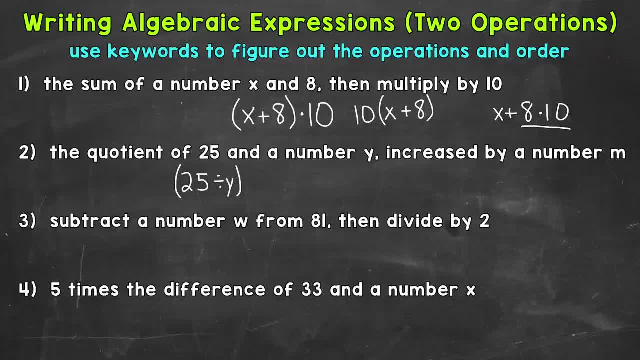 Increased is our key word, And this means that we are going to add M, So plus M, And that's our algebraic expression. We can also write it without parentheses, though, because due to the order of operations, we need to do division. 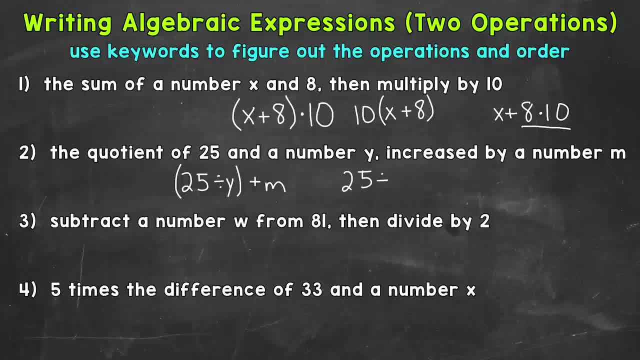 before addition. So 25 divided by Y plus M would be correct as well, Again, because due to the order of operations we need to do division before addition. So we would have to do 25 divided by Y first and then add M. 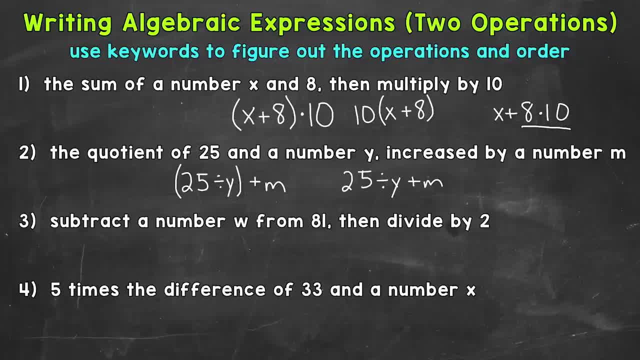 Let's move on to number three, where we have subtract a number- W from 81, then divide by two. So we need to subtract W from 81 first. So 81 minus W We are taking W from 81. So we switch that order there. 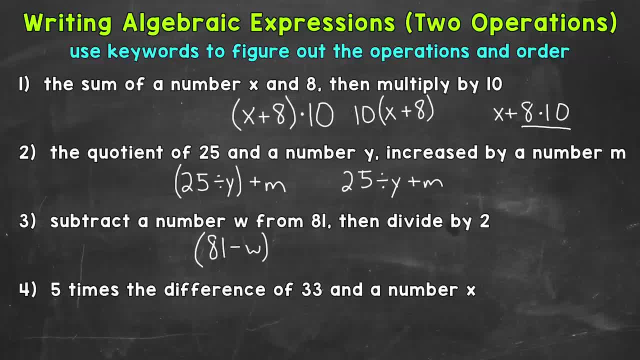 And I'm going to put it within parentheses to show that that is what we need to do first. Then we divide by two. So divide by two. Now, another way we can write this: we can do 81 minus W. put that in parentheses. 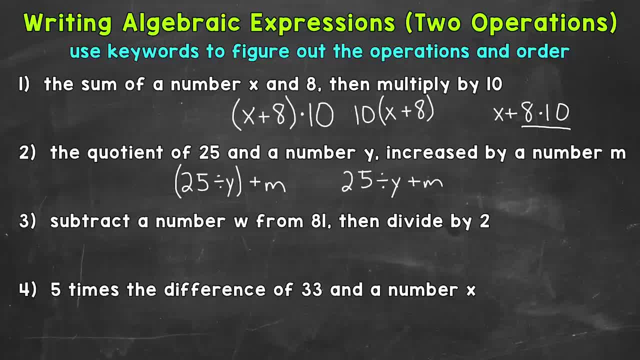 So we need to subtract w from 81 first. So 81 minus w, We are taking w from 81. So we switch that order there And I'm going to put it within parentheses To show that that is what we need to do first. 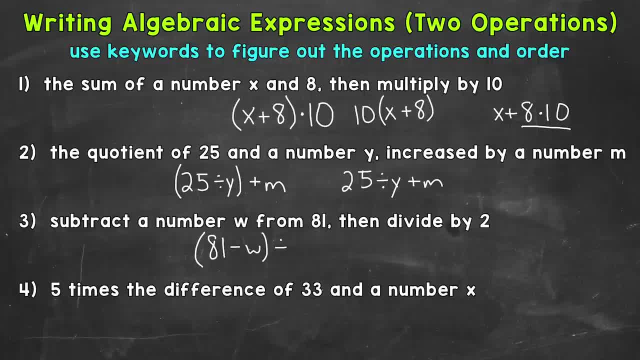 Then we divide by two. So divide by two. Now, another way we can write this. We can do 81 minus w, Put that in parentheses, And then we are going to write this as a fraction. So 81 minus w, in parentheses, over two. 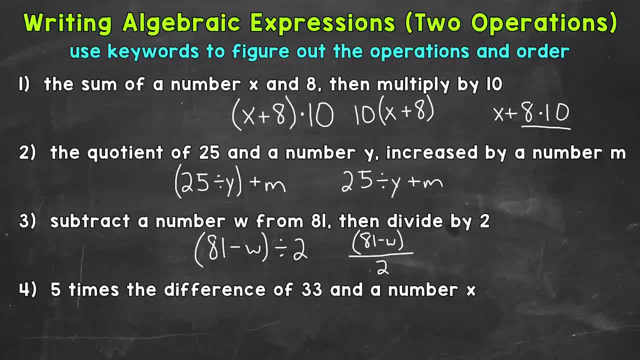 That represents division as well. So something to keep in mind. Lastly, Number four, We have five times the difference of 33 and a number x, So we need to find the difference of 33 and x And then multiply that by five. 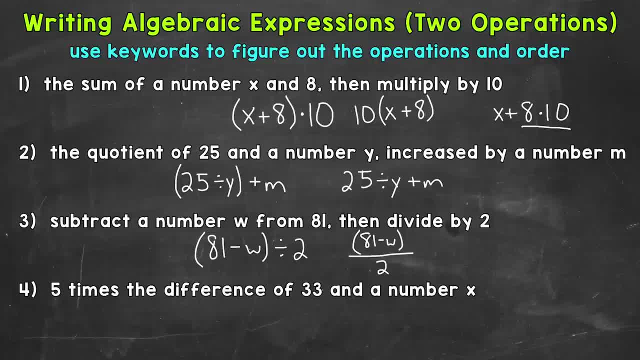 So we need to find the difference of 33 and x first. Difference is our keyword. It means the answer to a subtraction problem. So the first thing that we need to do Is find the difference of 33.. And then we have to find the difference of 33 and x. 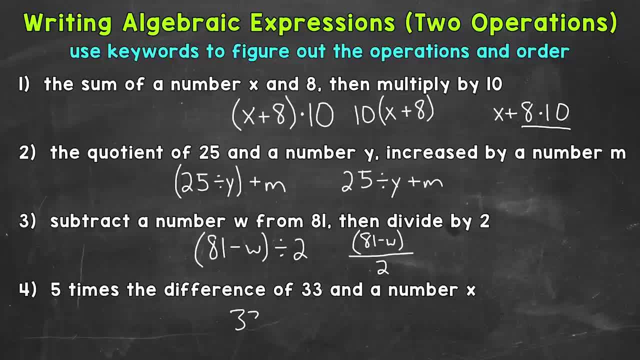 So 33 minus x, 33 minus x. Put that within parentheses here To show that that is what we do first, And we need to do five times that. So we can do five times that, Or we can do Five times that. 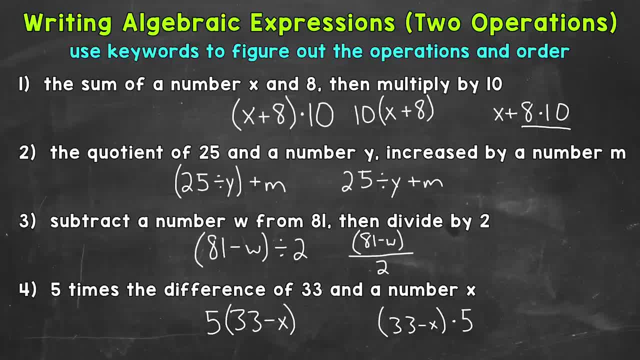 Afterwards, Afterwards. So 5 times the difference of 33 and a number x. I would highly suggest, after you write out your algebraic expression, double or even triple, check it with that original phrase to see if they match. So there you have it. 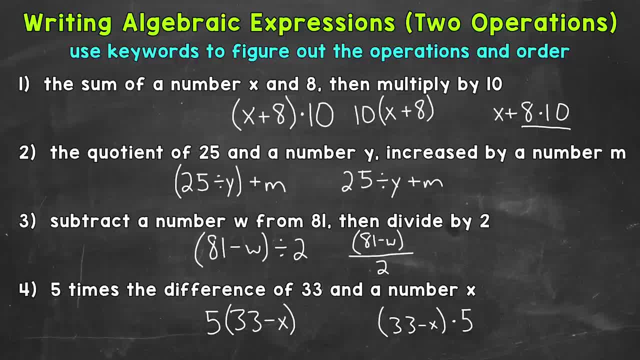 There's how you write algebraic expressions. I hope that helped. Thanks so much for watching. Until next time, peace.